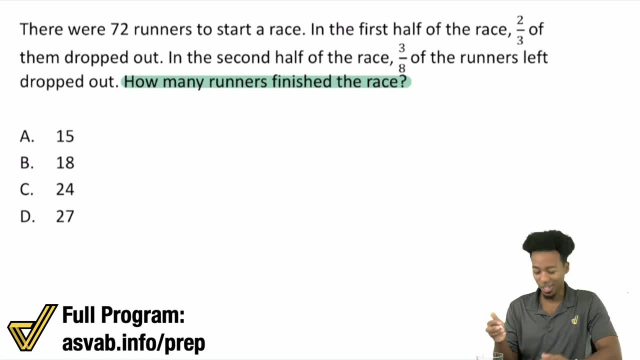 might not always be obvious, but we at least know what we're looking for. And that's right there: The runners that finished the race. So let's write that down, Number one again, what we want. we want to know: hey, how many finished the race? So in a sentence we can say: blank runners finished. 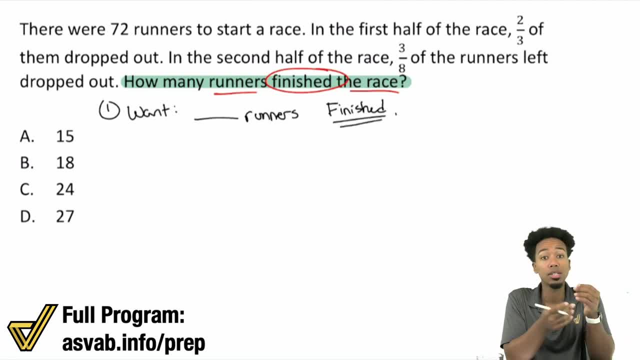 Okay, So there's an emphasis on the word finished because, again, when we take a look at the problem, there might be information that talks about people dropping out, people going on, people finishing right. So we want to make sure that we gear our attention toward those who finish. That way we don't get distracted. 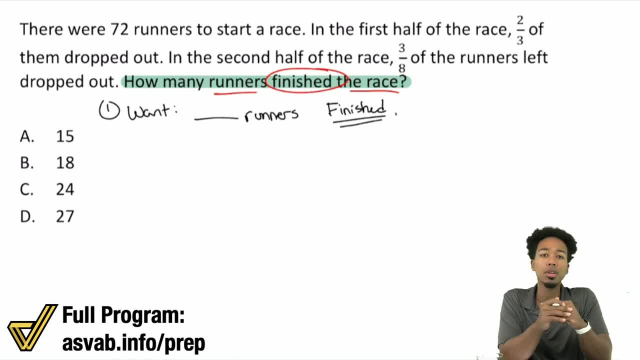 So step two, it's going to be: hey, let's go ahead and just sort through the information, sort through the story and see what these numbers mean in terms of what they give us. Let's go and check it out. So here we see that there were 72 runners to start a race. 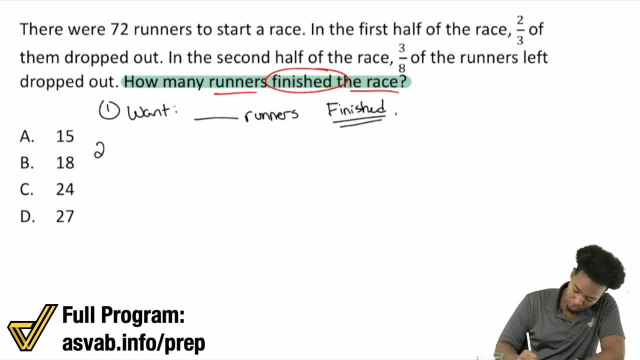 Okay, So let's write that down. So again, step two: the information that we have- we have 72 started, 72 started- Sounds good, So let's go ahead and highlight that. Then, from there, it says hey, in the first half of the race. 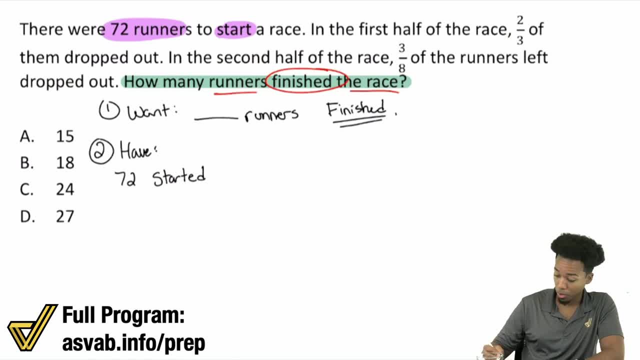 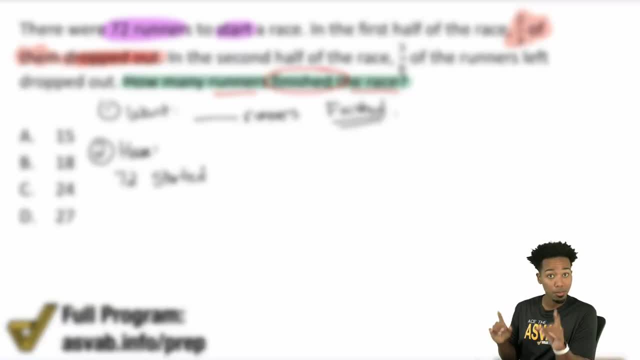 two thirds of them dropped out. Okay, So that's really important there, right, Two thirds of them dropped out. As always, my MazVap party people, thank you for watching this video Before we continue. just wanted to remind you that if you're struggling with the ASVAB, if you struggle with 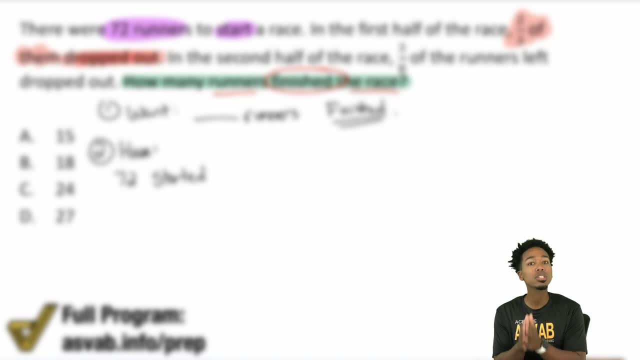 test anxiety, blanking out on problems, then you need to consider the ASVAB All Access program. Thousands of my students have tried it out and they have always raised their scores, if they use it the right way, because there's always a way to learn for whatever method you like best. 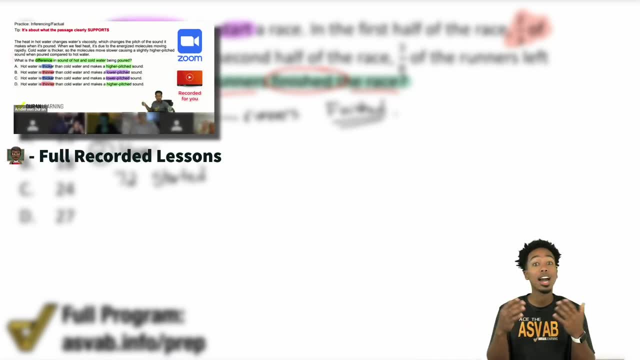 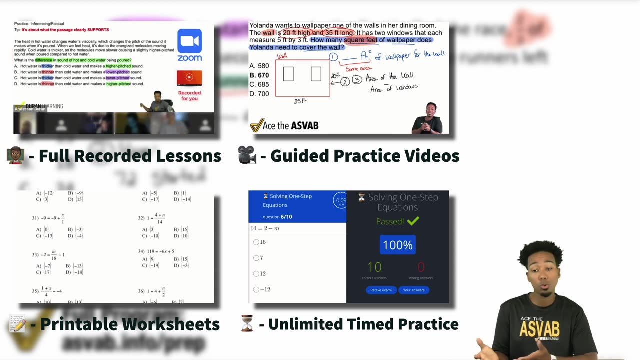 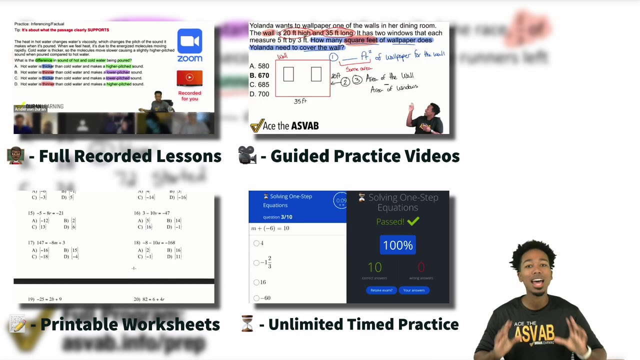 from recorded lessons to live classes, to guided practice videos, to printable worksheets, to speed drills to help you test and raise your confidence in speed, to casual practice. that comes with video solutions- Every single way that you can think of. over 10,000 questions. all of it lined. 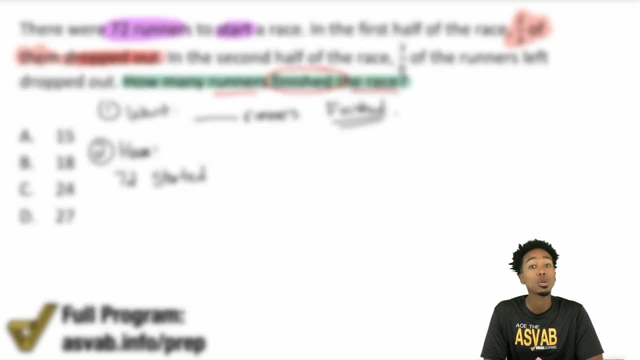 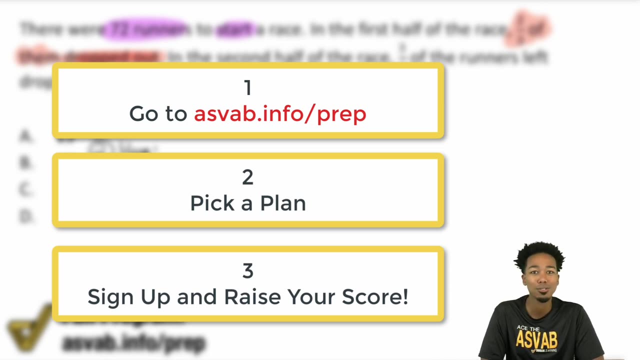 up for you, ready for you to get started right now. So, at the very least, check out the link in the description so you can see exactly how it works and why. again, over a thousand of my students have raised their scores with it all the way through. I'm proud of you. Let's keep working hard. 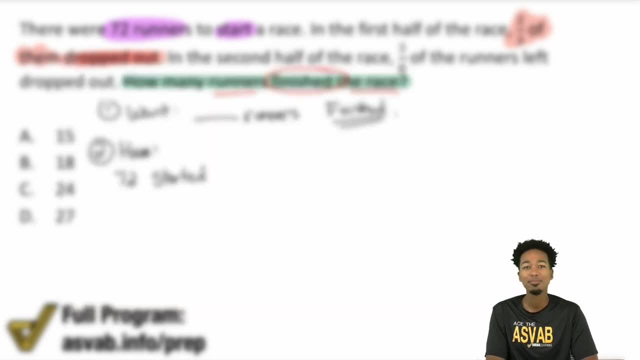 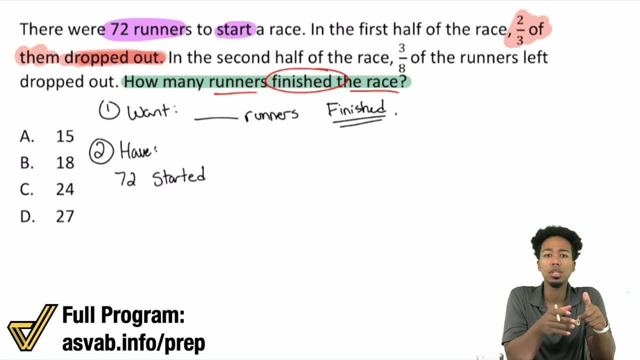 and let's get back to the video, But don't forget, check out that program. I think you'll like it Dropped out, Okay? So what does that mean? Well, this is where it's really important to understand how fractions work. Remember that when it comes to fractions, 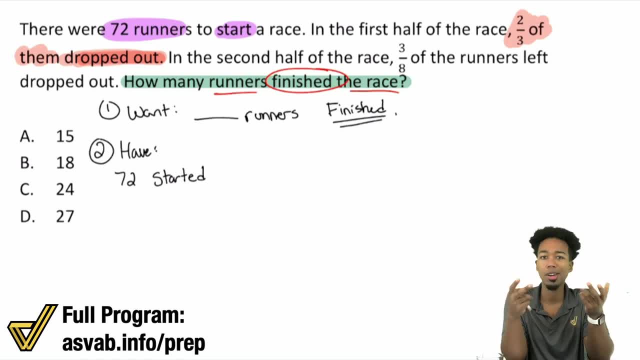 fractions are always going to be parts of wholes- right, Parts of wholes- And what that really means is, when you have the same number on top as the bottom, you have the whole thing. So this is where a lot of us might get confused. This is one way to do the problem. There are plenty of other ways. 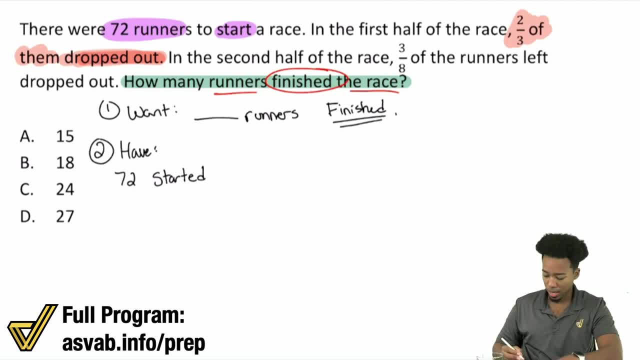 I'll show you two ways here. The one way to do this is to understand that hey look, if two thirds of them dropped out. that means, and think about it like this: if two thirds dropped out, well, how many are left? 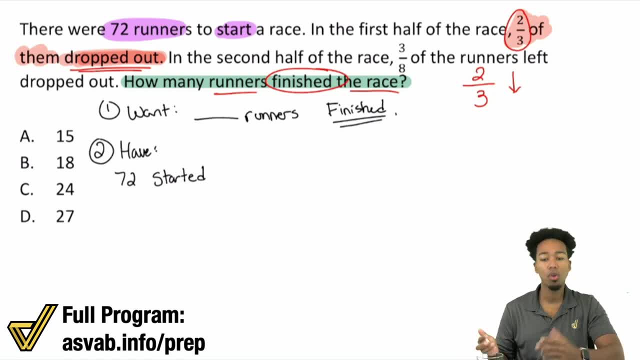 One third. Remember, fractions are parts of wholes. The whole thing is out of three. So if we have two out of three, we have one left out of three. So if two thirds drop out, one third remains, stays or continues. Okay, Let's go ahead and understand how that makes sense. Fractions are: 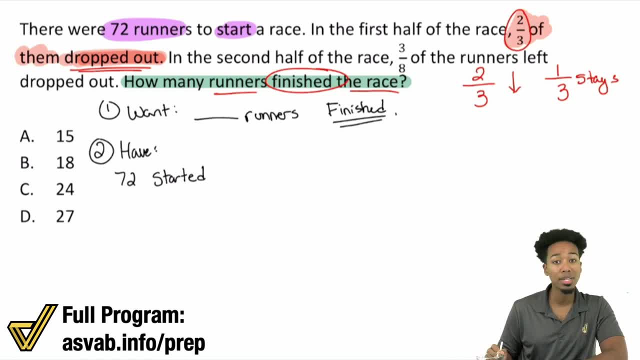 parts of wholes. So if we have two out of three dropping out, one out of three stay, Because two plus one that would make the whole three out of three. Way too important to understand that. my math party people Way too important. So why do I want to know how many stay? 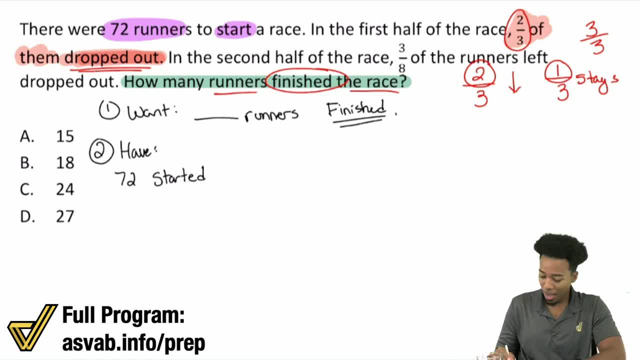 Because we have to pay attention to the question. The question said: how many finished? So do we want to count up how many people dropped out? No, we want to count how many people stayed. 72 started. Then we have one third left of the 72. So of those 72 people that originally started, 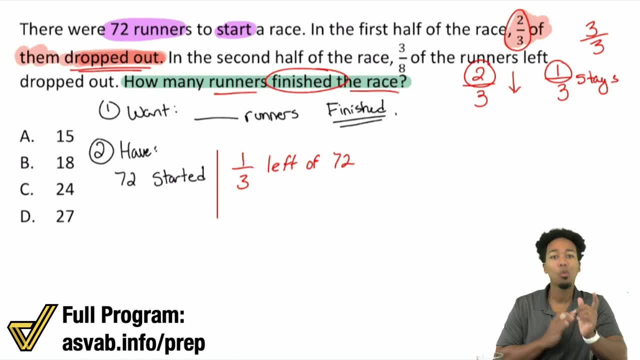 we have one third that stayed, Again, two thirds dropped out, one third stayed. And then what happens next? Let's see, Let's understand what happens next. It says here: in the second half of the race, three eighths of the runners left dropped out. So three eighths of the runners that are left. 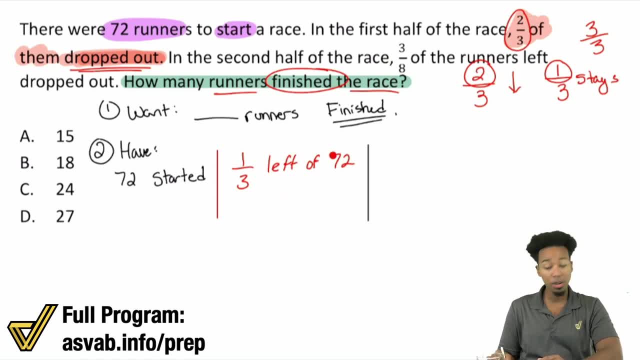 so after this, one third are left, you know whatever number that is. whatever number that is, three eighths of them dropped out. So what does that mean? So if three eighths dropped out, well, think about it again. Fractions are parts of wholes. So if you have three out of eight, 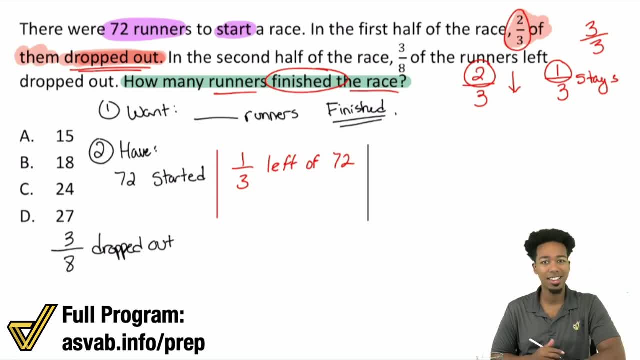 dropping out, five out of those eight, stay. Five of those eight people stay, Because again, three plus five would make the eight out of eight. right. So five out of eight stay. Or in this case, finish, right. So here, five eighths stay, slash, finish. 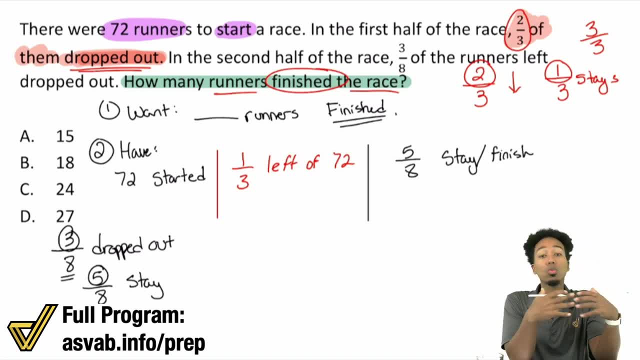 So, before I even do the math, I understand what route I'm going to take, Since I want to know how many runners finished. guess what? Hey look, 72 started. A third of those people were left after the first half, And then whatever number. that is, a third of 72, whatever number that is. 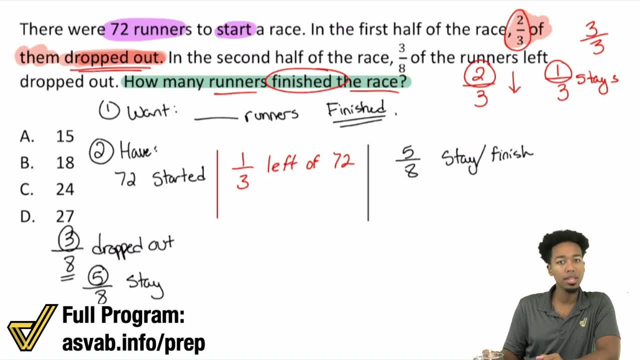 then five, eighths of those people that are left. they finished, And there's our answer. So, now that we have the plan set up, let's dive on in and we're good to go. So right here. what's a third of 72? Well, one third of 72, that's going to go ahead and be what? 24.. 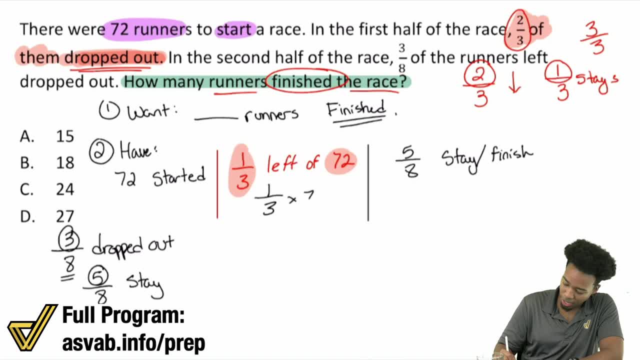 So the way that we calculate a third of 72, that's the same thing as saying one third times 72, which is the same thing as saying 72 over three, Same thing as saying 72 over three. And if we divide three into 72, we get two. Two times three is six. so we have one left. Drop that two. 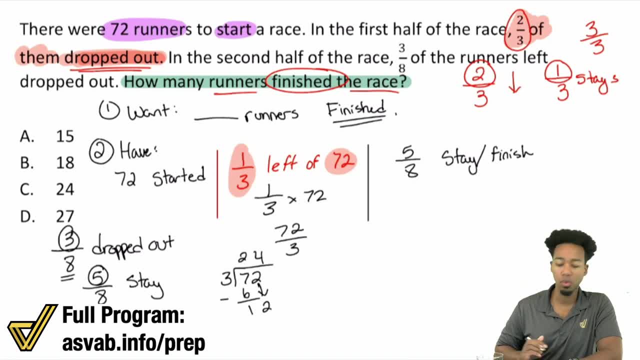 so three into 12, that's four, a very even four. So that means that we have again 24 that are left. So where does that go? Right there, Five eighths of the 24 people. those are the people that finish. So five eighths of 24,. 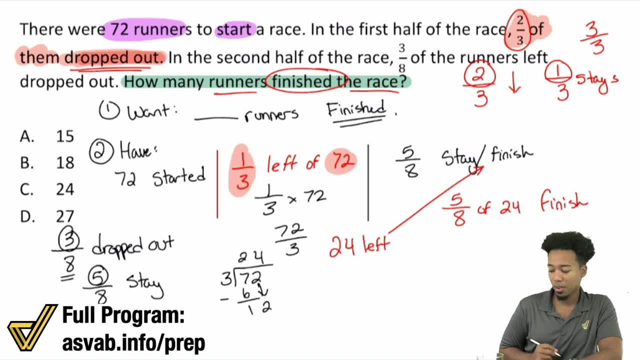 finish the race. You're not done yet, because now we need to do five eighths of 24.. So that's going to be over here: five over eight times 24, which is the same thing as saying 24 over one. 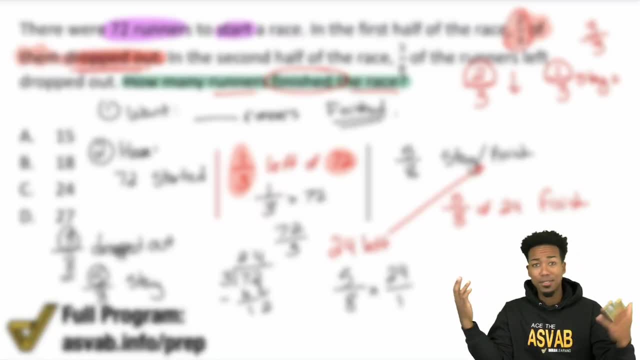 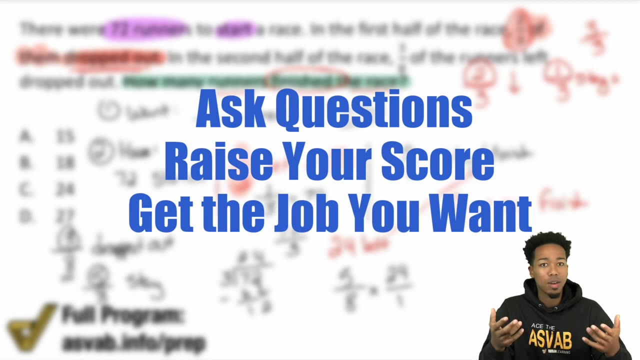 Same thing, And so whether this is your first or 50th YouTube video of mine, it doesn't matter. Why don't you join me for a live class? That way, you can ask questions, raise your score and get the job you want for free Again. I host classes once a week on Zoom. 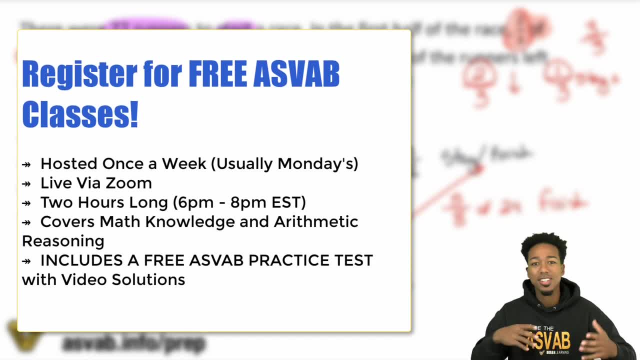 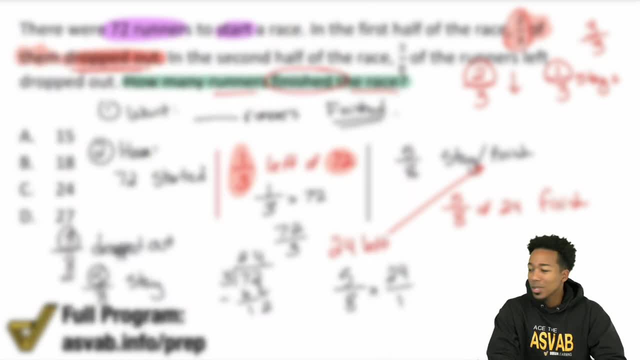 typically on Mondays. So go ahead and click the link up there down here somewhere. register for free and you get my free practice test that has video solutions so you can learn from every mistake. That's what it's all about here. my party people. 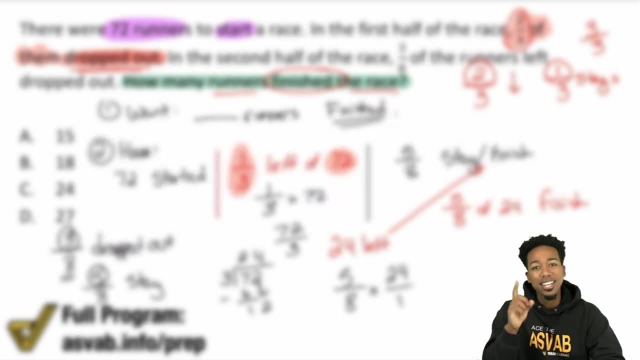 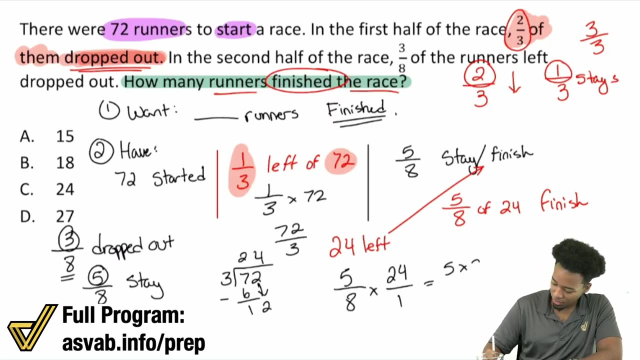 I want to help you succeed, so don't hesitate, Sign up for free, and then let's get back to this problem here. Let's keep raising our scores, And here we can say that that's five times 24 over eight. The reason I wrote it like this is because this is going to be a little easier, for 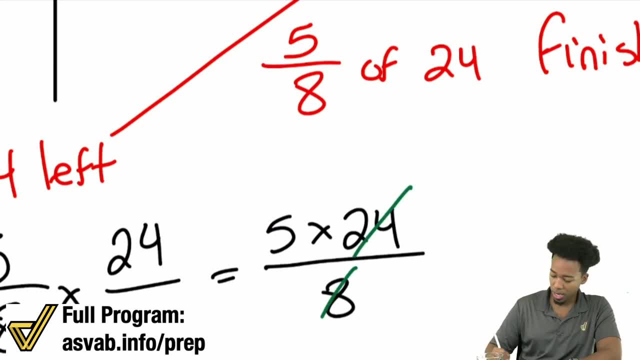 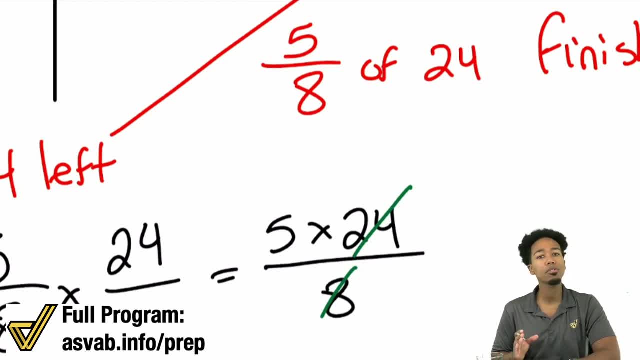 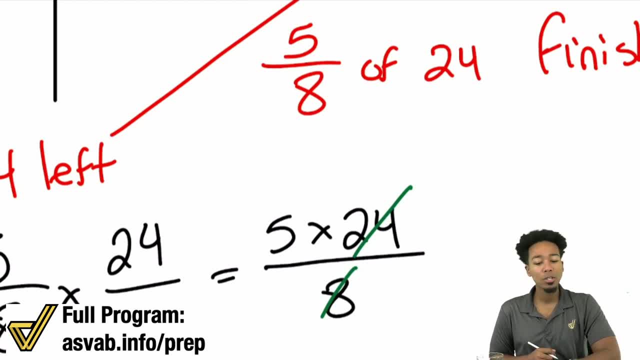 because again, you're gonna deal with easier numbers here. And so there, 24 divided by 8, that's the same thing as saying 3 over 1.. Because, again, 24 and 8 are both divisible by 8.. 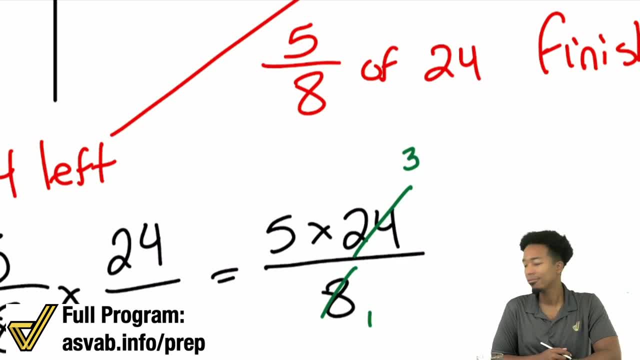 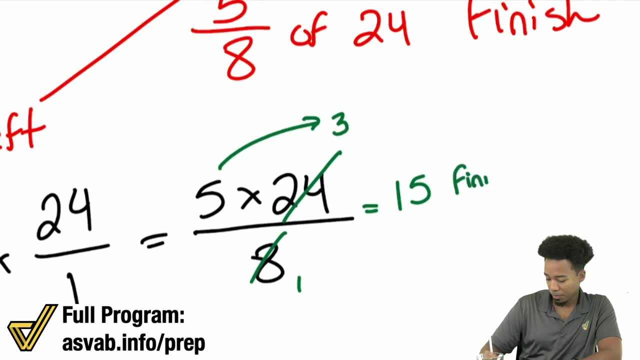 24 divided by 8 is 3.. 8 divided by 8, 1.. So now all we have is 5 times 3,, which is 15, and it's 15 runners finished, And so I want to review. 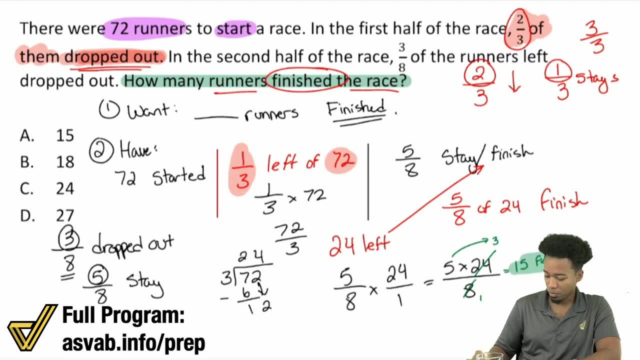 And so I want to review. And so I want to review this one more time for us here, because again we have the answer: 15 runners finished. but i want to make sure you understand that if you took the route of saying, hey, let's go ahead and do the 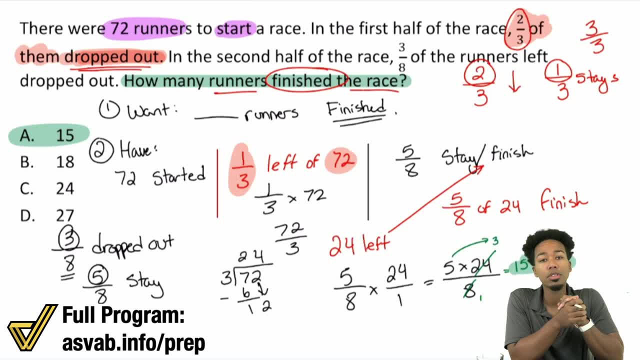 two-thirds of 72. if you did the two-thirds of 72, you would have gotten 48 and with that 48. you need to understand what that number means, because if you would have gotten 48 in the beginning, that's 48 runners that dropped out. and guess what? if you would have done 72 minus 48, that's the 24 that are.